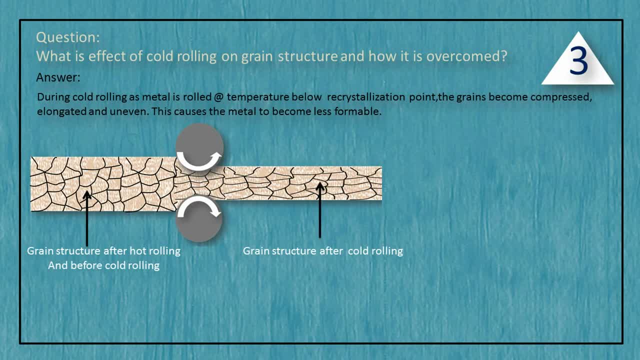 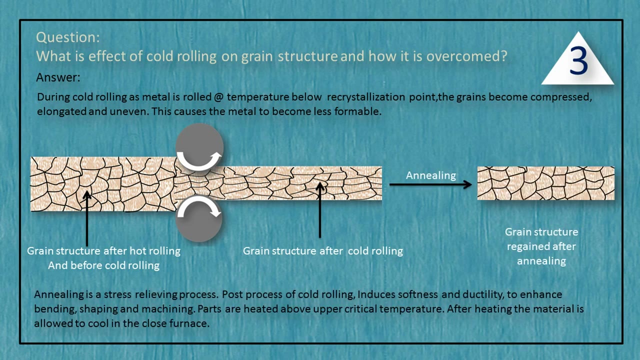 And how it is overcommed. Answer: During cold rolling. as metal is rolled at temperature below recrystallization point, the grains become compressed, elongated and uneven. This causes the metal to become less formable. Annealing is a stress relieving process. 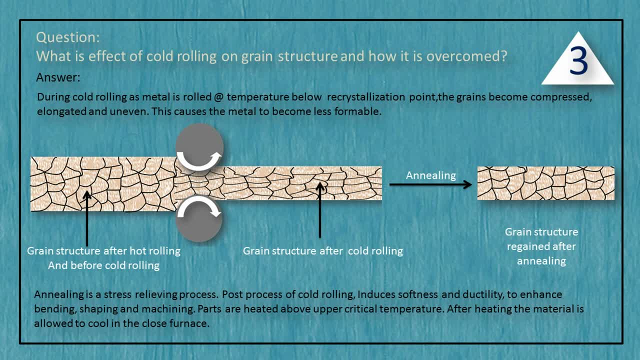 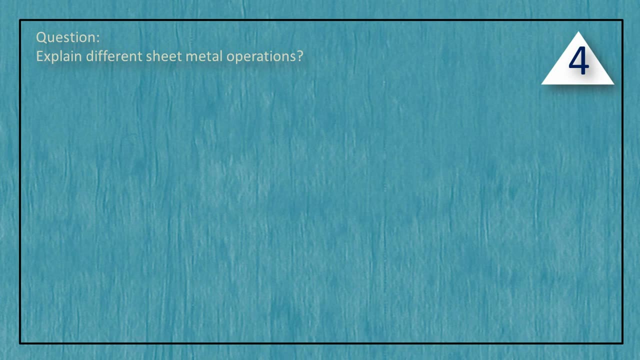 Post. process of cold rolling induces softness and ductility. to enhance bending, shaping and machining Parts are heated above upper critical temperature. Answer: After heating, the material is allowed to cool in the close furnace. Question: Explain different sheet metal operations? Answer. 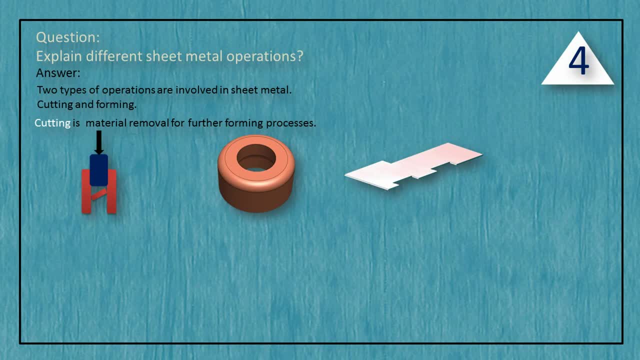 Two types of operations are involved in sheet metal: Cutting and forming. Cutting is material removal for further forming processes. Answer: The cutting is for giving a particular shape to sheet or making certain designs on the sheet's surface without material removal. Question. 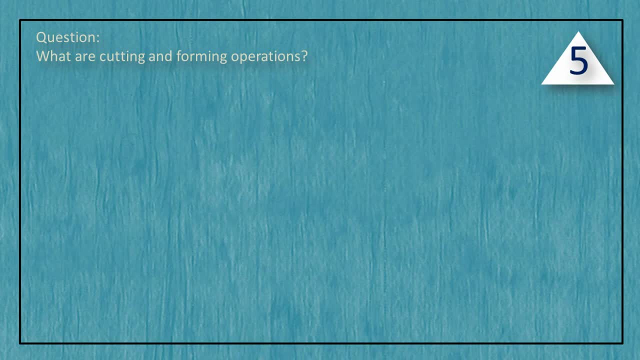 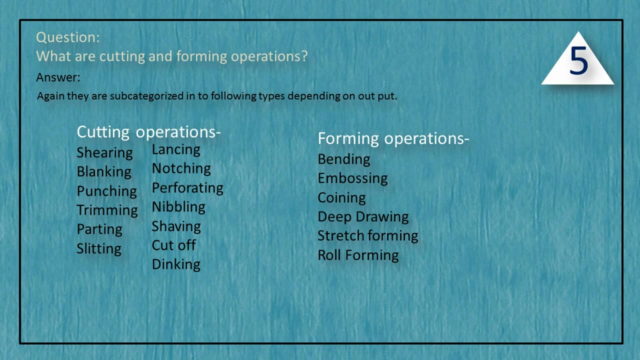 What are cutting and forming operations? Answer: Again, they are subcategorized into following types, depending on output: cutting operations shearing, blanking, punching, trimming, parting, slitting, lancing, notching, perforating, nibbling, shaving, cutoff and dinking. and forming operations are bending, embossing, coining, deep drawing, stretch, forming and roll. 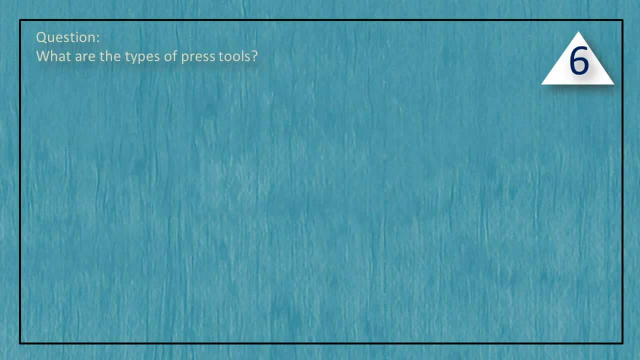 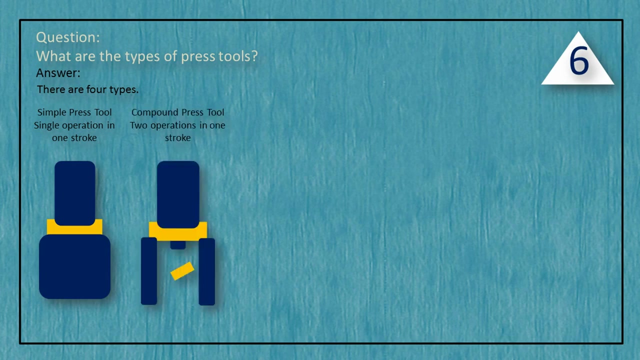 forming question. what are the types of press tools? answer: there are four types: simple press tool- single operation in one stroke. compound press tool- two operations in one stroke. progressive press tool: keeps moving the sheet metal to subsequent stations after each stroke. combined press tool- two operations in one stroke at two. 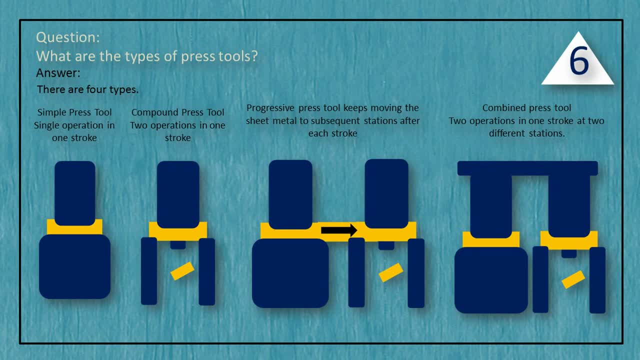 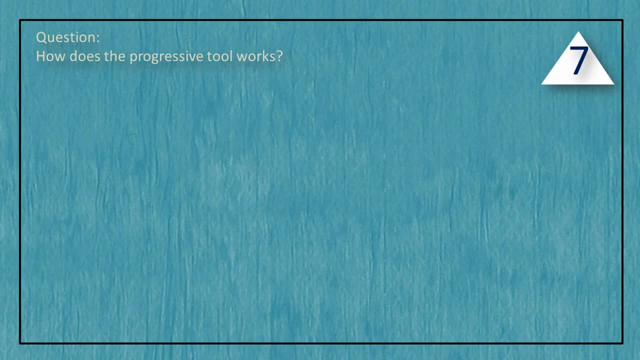 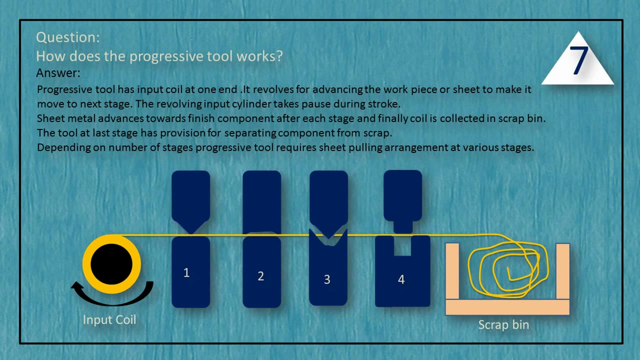 different stations. question: how does the progressive tool works? progressive tool has input coil at one end. it revolves for advancing the workpiece, a sheet to make it move to next stage. the revolving input cylinder takes pause during stroke. sheet metal advances towards finish component after each stage and finally coil is collected in scrap bin. the tool at last stage has 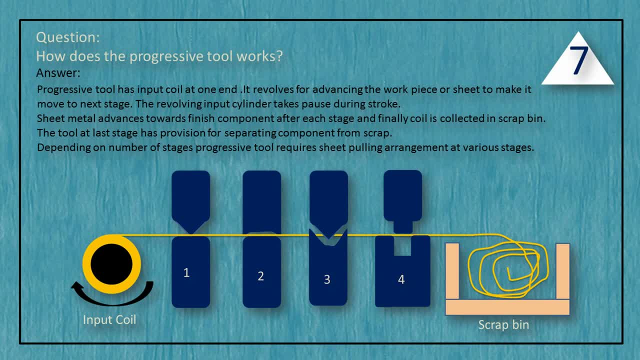 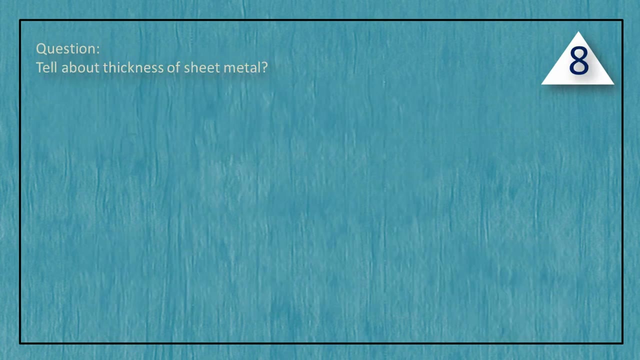 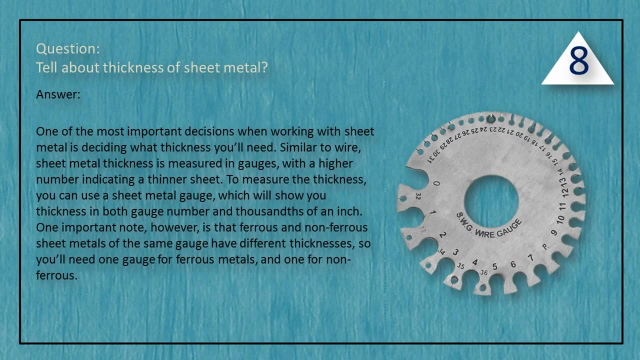 provision for separating component from scrap depending on number of stages. progressive tool requires sheet pulling arrangement at various stages. question tell about thickness of sheit metal. answer. one of the most important decisions when working with sheath metal is deciding what thickness you'll need. similar to wire sheat Heightage. 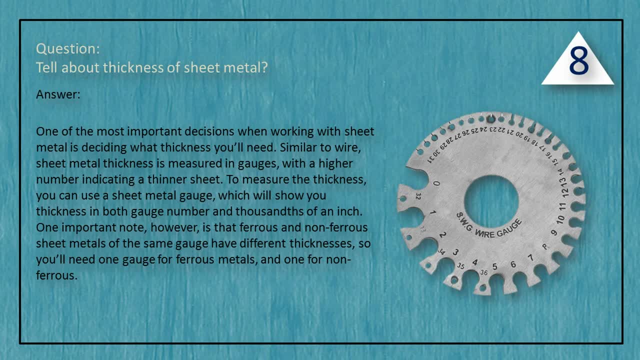 The sheet metal thickness is measured in gauges, with a higher number indicating a thinner sheet. To measure the thickness, you can use a sheet metal gauge, which will show you thickness in both gauge number and thousandths of an inch. One important note, however, is that ferrous and non-ferrous sheet metals of the same gauge have different thicknesses. 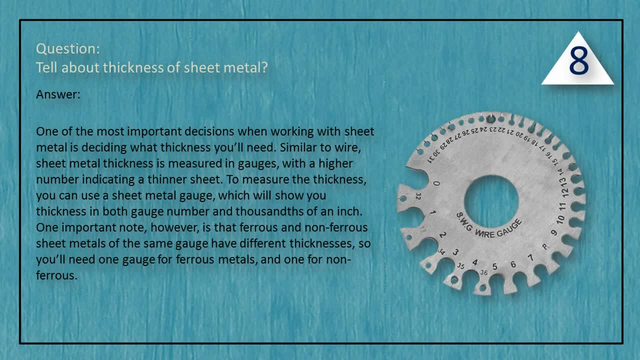 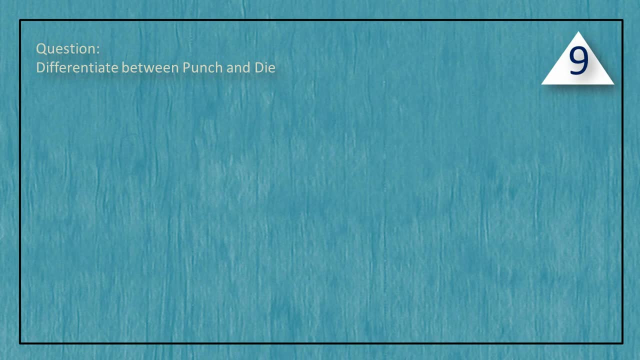 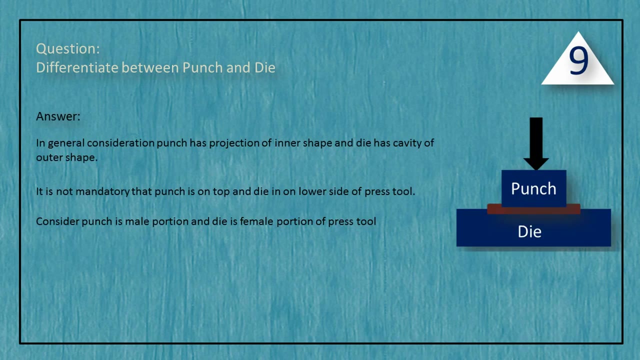 so you'll need one gauge for ferrous metals and one for non-ferrous. Question: Differentiate between punch and die. Answer: In general consideration, punch has projection of inner shape and die has cavity of outer shape. It is not mandatory that punch is on top and die in on lower side of press tool. 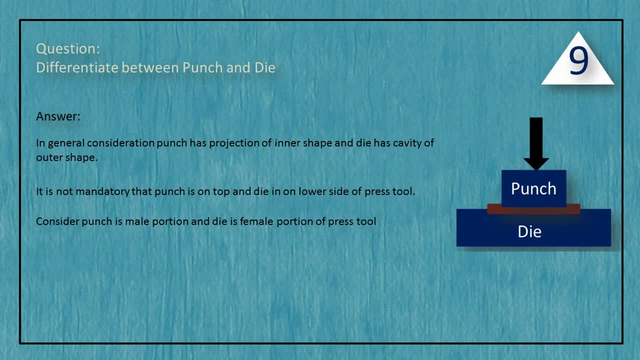 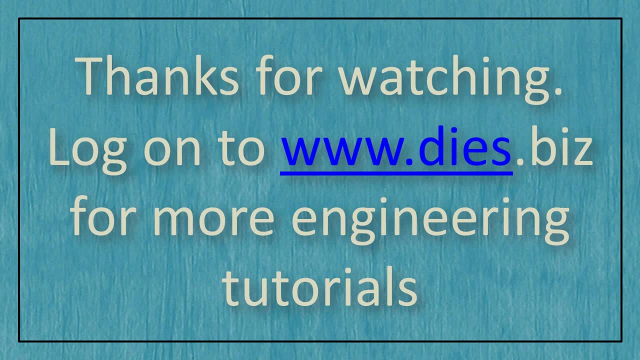 Consider: punch is male portion and die is female portion. This is female portion of press tool. Thanks for watching. Log on to diesbiz for more engineering tutorials.